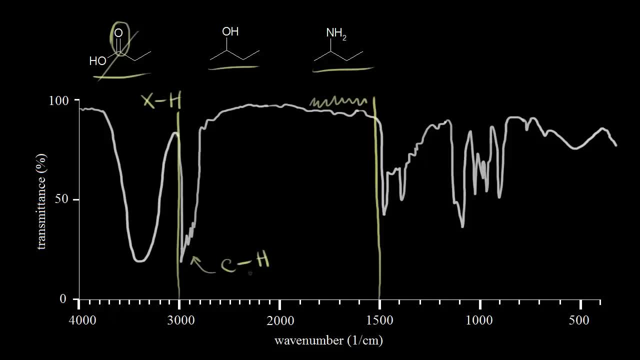 and I know below that we're talking about a carbon-hydrogen bond stretch where you have an sp3, hybridized carbon. That doesn't help us out here at all, but this other signal does. So we have another signal, so it's centered on a higher wave number. 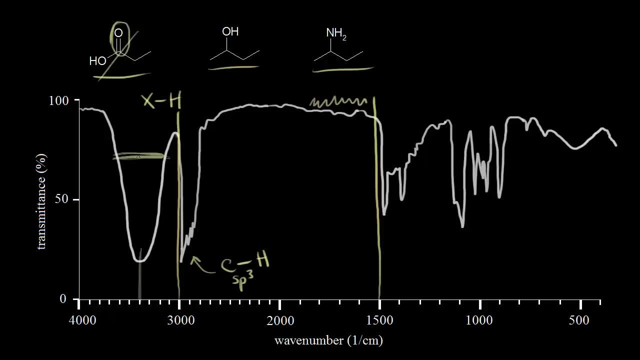 and it's extremely broad. So whenever you see that, you should think to yourself: hydrogen bonding and this is due to an OH bond stretch, So immediately we know that we must be talking about an alcohol here. A carboxylic acid has a similar OH bond stretch. 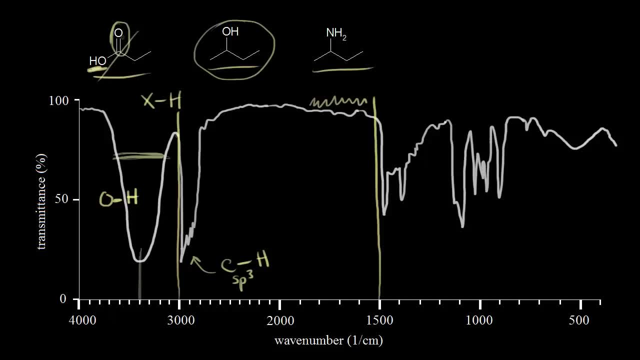 so it has a broad signal due to that, but there's no carbonyl, so it couldn't possibly be this molecule. It also couldn't possibly be the amine because, even though we have nitrogen-hydrogen bond, a nitrogen-hydrogen bond stretch. 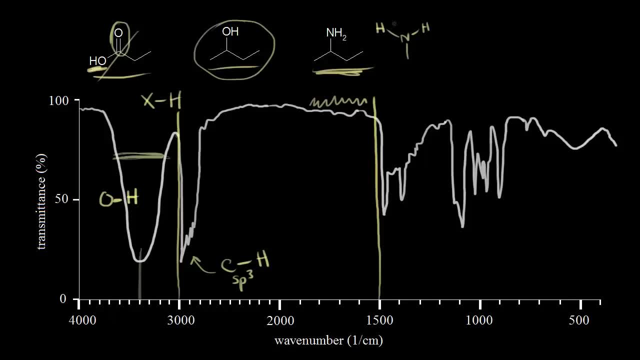 is going to be in a similar region. we would expect two signals for this. We would expect a symmetric stretch signal and an asymmetric stretching signal, and it wouldn't be as broad as what we're talking about here for the alcohol. so it's definitely not the amine. 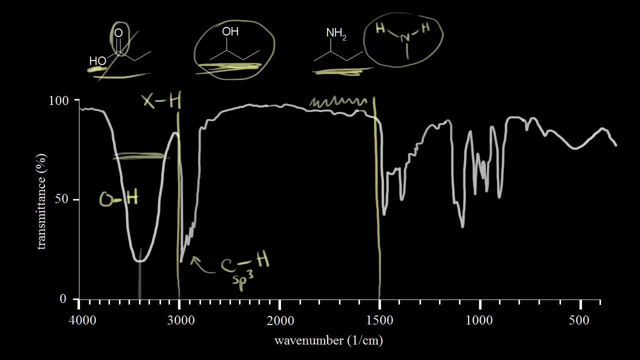 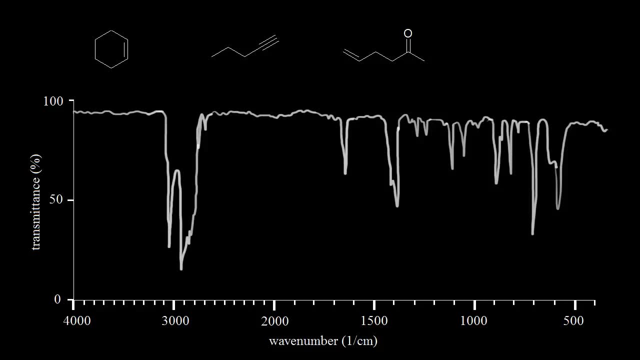 So this spectrum is the alcohol. Let's look at three more molecules in a different spectrum. So let's look at the spectrum. here We start with 1,500.. So we draw a line. here We look in the double bond region. 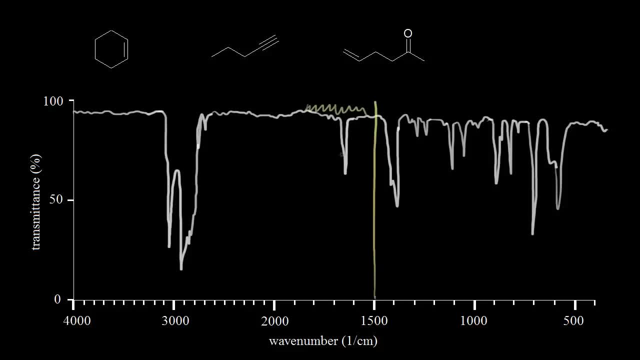 So here's our double bond region. I do see a signal this time, and it doesn't look like it's a very strong signal either. Let's see what the location of this signal is. So I drop down and the signal shows up between 1,600 and 1,700. 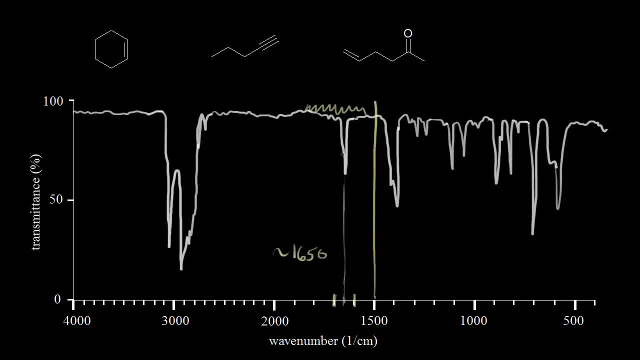 So we'll say approximately 1,650.. That's not very strong. Both of those things- the location and the fact that it's not a very strong signal- clue me into the fact that this is probably a carbon-carbon double bond stretch. 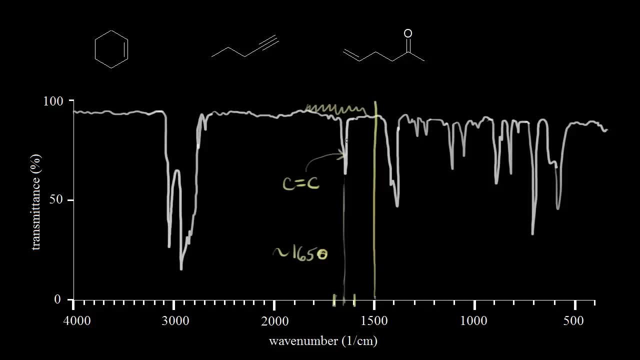 That's what this is talking about here. So a carbonyl. we would expect that to be just past 1,700 and also much, much stronger. So we can rule out this molecule over here, because I don't see any kind of a carbonyl stretch. 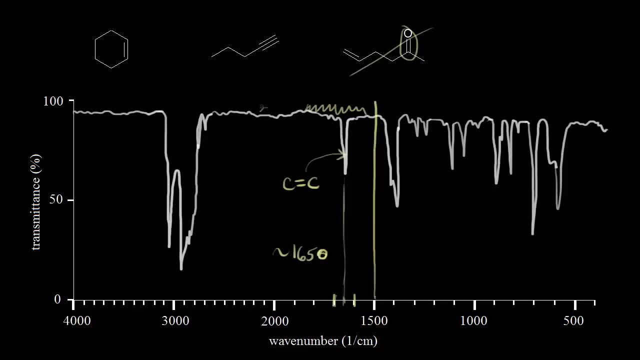 So let's look in the triple bond region. So somewhere in here I don't see any kind of a signal here, So it couldn't possibly be this molecule. So we must be talking about cyclohexene here. And if we look over in the bond to hydrogen region, 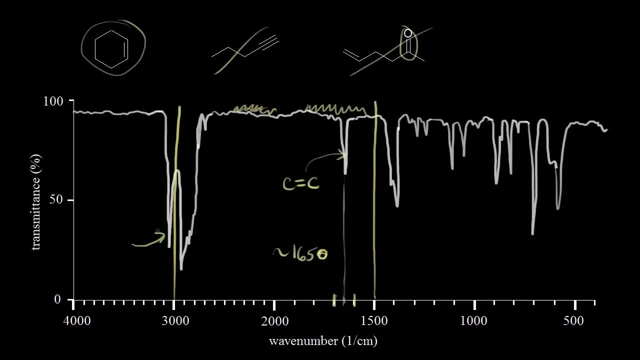 and we draw a line, we can see that this signal just higher than 3,000,. this must be talking about our carbon-hydrogen bond stretch, where the carbon is sp2 hybridized. So this is, of course, talking about our carbon-hydrogen stretch. 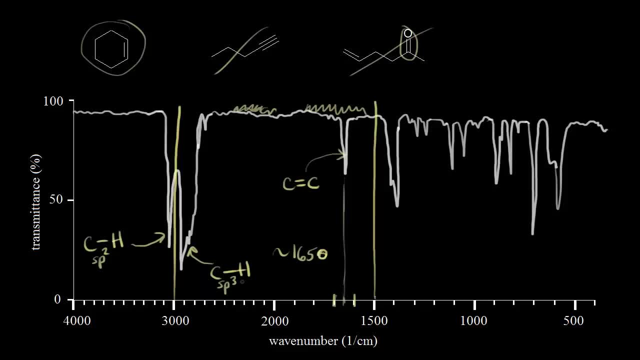 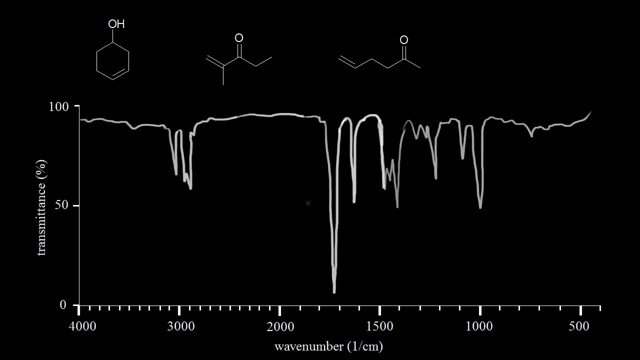 where we're talking about an sp3- hybridized carbon- And so cyclohexene is the only thing that makes sense with this IR spectrum. Let's do one more, So we have three molecules and an IR spectrum, All right, So let's start analyzing. 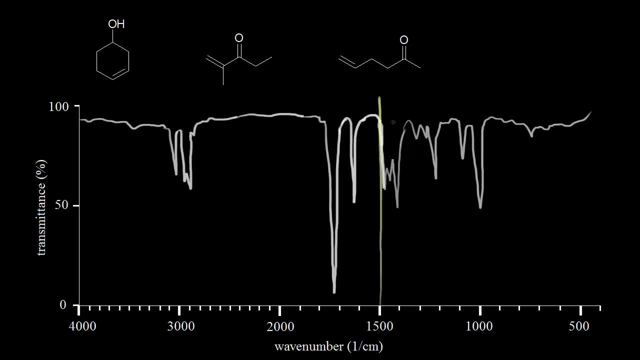 Draw our line around 1,500 right here, Focus in to the left of that line, And this is our double bond region. So two signals, two clear signals in the double bond region. Let's look at this signal right here. All right. 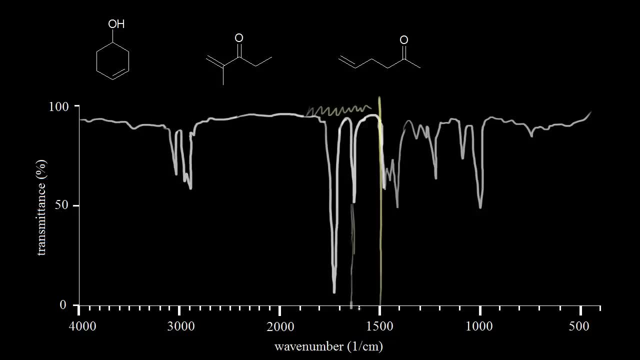 So this is not as intense as the other one And it's pretty much between 1,600 and 1,700.. So both those factors make me think carbon-carbon double bond stretch. So this is probably a carbon-carbon double bond stretch here. 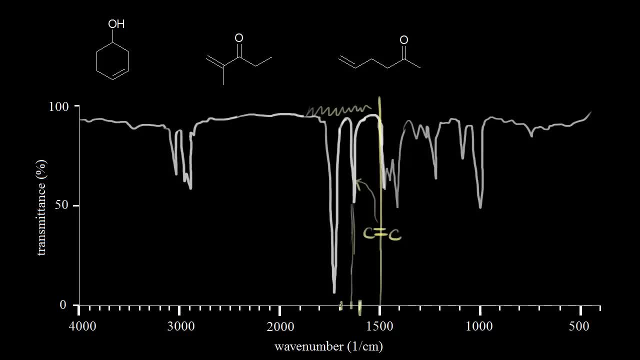 The signal next to it. if this is 1,600, this is 1,700. So this signal is just past 1,700. And it's very strong. It's a very strong signal. So that makes me think carbonyl. 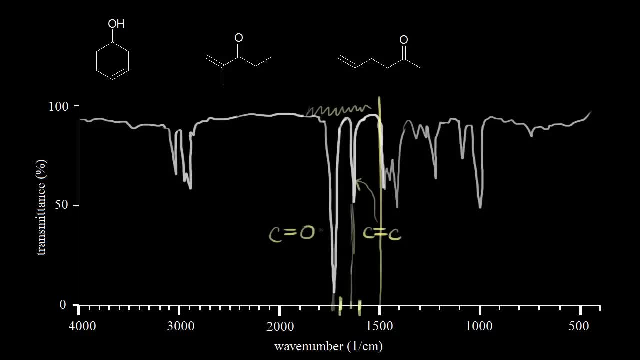 All right, So this makes me think carbonyl right here, So we can immediately rule out this one. All right, So it couldn't possibly be that molecule. And that brings us to this, which is a conjugated ketone versus an unconjugated ketone. 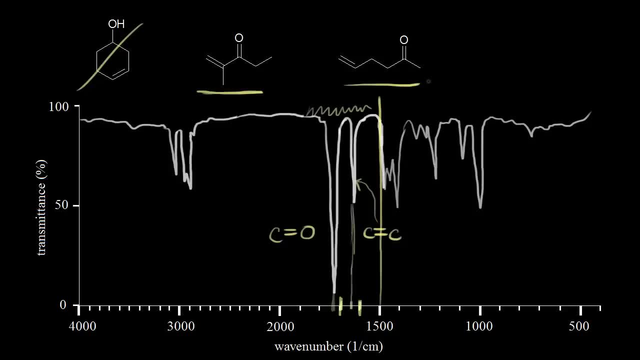 All right. So let's think about the unconjugated ketone for a minute here. So this carbonyl stretch we talked about in an earlier video. we'd expect to find that somewhere around 1,715.. So past 1,700..